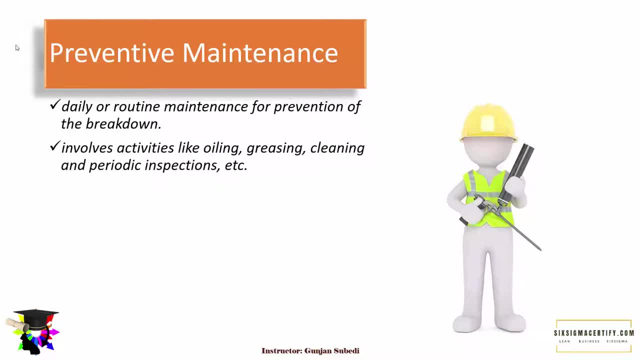 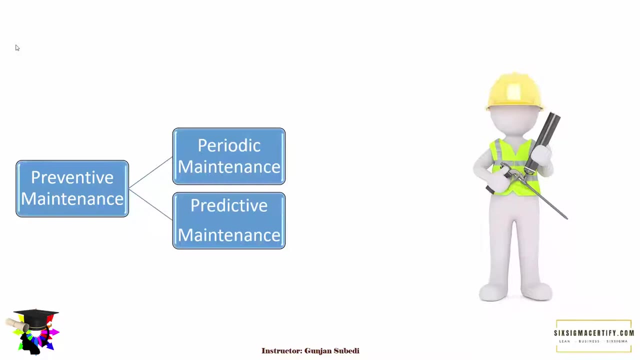 and periodic inspections, etc. Preventive maintenance extends the life of any equipment or machines. There are basically two types of preventive maintenance: Periodic maintenance and predictive preventive maintenance. So what is periodic maintenance? Periodic or time-based maintenance involves activities such as inspection, cleaning and servicing or replacing the defective parts of the machine. 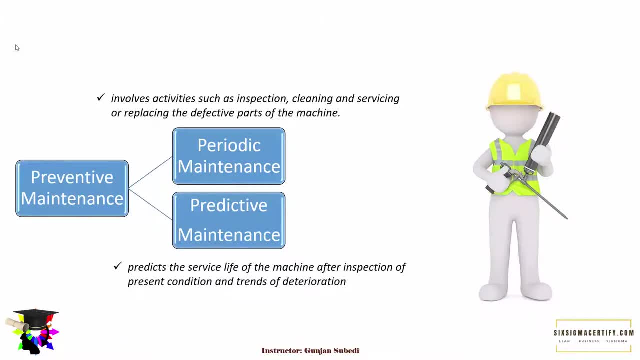 On the other hand, predictive maintenance is a condition-based maintenance in which we predict the service life of the machine after inspection of the present condition and trends of the deterioration, so that with maintenance activity it also employs the surveillance system of the condition of the machine. 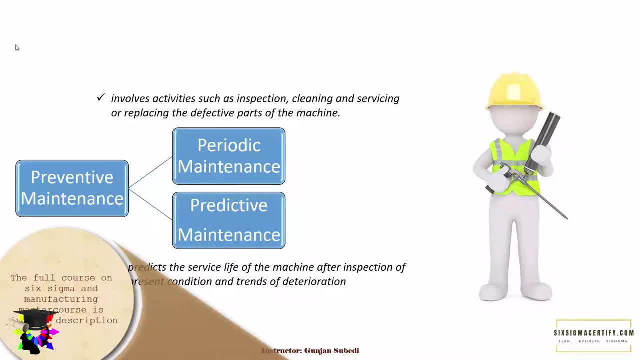 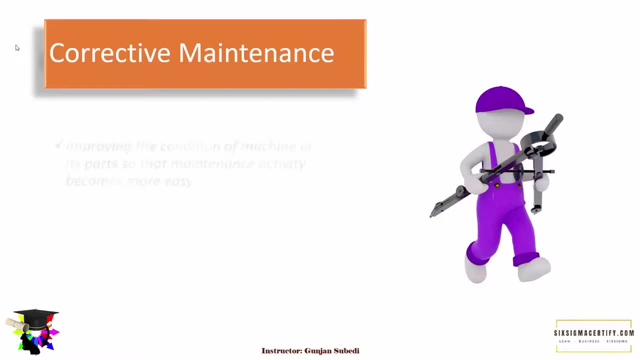 So that is predictive maintenance. There is another type of maintenance, There is another type of maintenance, There is another type of maintenance called corrective maintenance, And this is basically primed at improving the condition of the machine or its parts so that the maintenance activity becomes more easy. 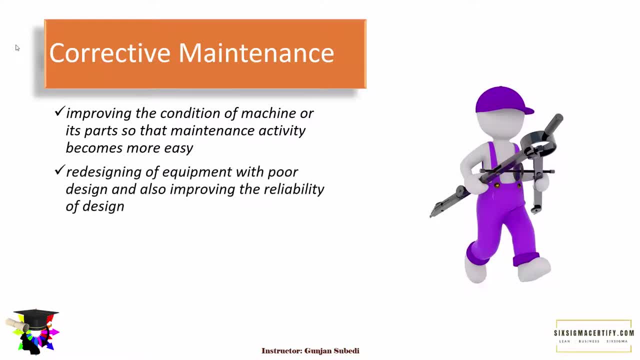 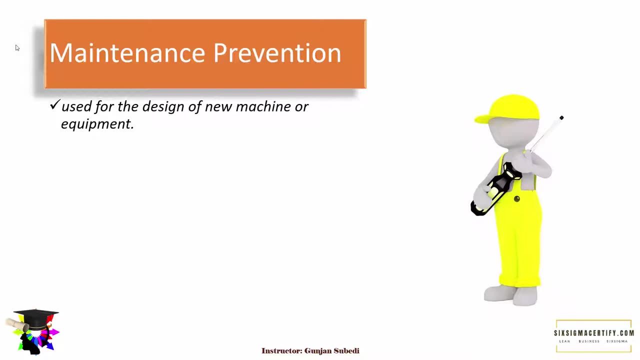 Basically it can include redesigning of the equipment with poor design and also improving the reliability of the design. And the last one is maintenance prevention, which is basically used for the design of the machine, The design of new machine or equipment. For this, the weakness or drawbacks of the current machine is studied and the features of improving the safety, working efficiently, making it more easy for future cleaning and maintenance, etc. are added to the machine. 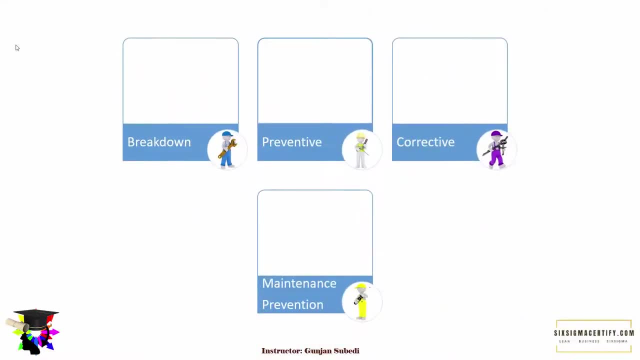 So basically, we studied four types of maintenance. Some of these may be important in some competitive exams like Lean, Six Sigma, Blackwell examinations, operations management and Kaizen certifications, etc. Even if you are not looking for any competitive exams, the quizzes and scenarios that I take could be helpful in understanding the concepts much better. 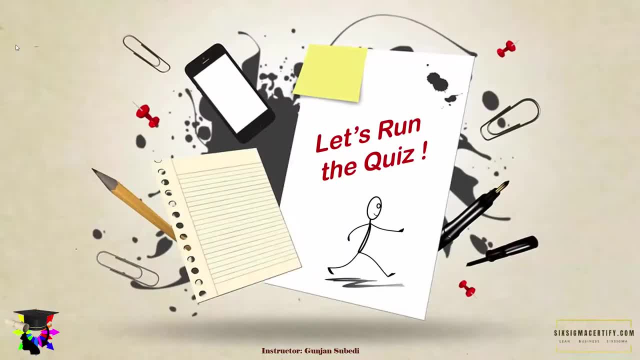 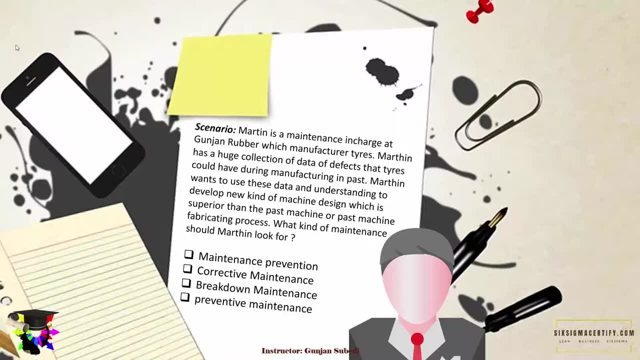 So, without further delay, let's run the quiz. Scenario: Martin is a maintenance in-charge as Gunzen Rubber which manufactures tires. Well, that's Gunzen Rubber. I could not think of anything while giving example than my own name. 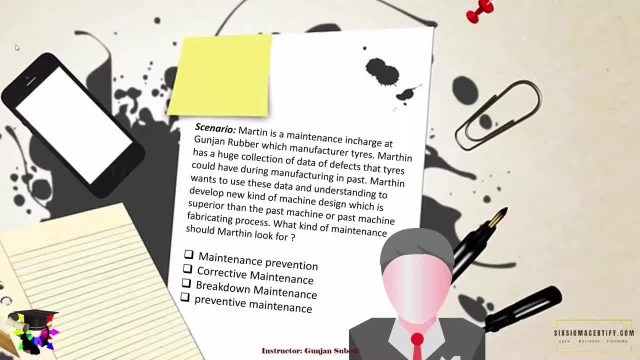 Sorry for that. Martin has a huge collection of data of defects that tires could have during its manufacture in the past. Martin wants to use these data and understanding to develop new kind of machine design which is superior than the past machine or past machine. 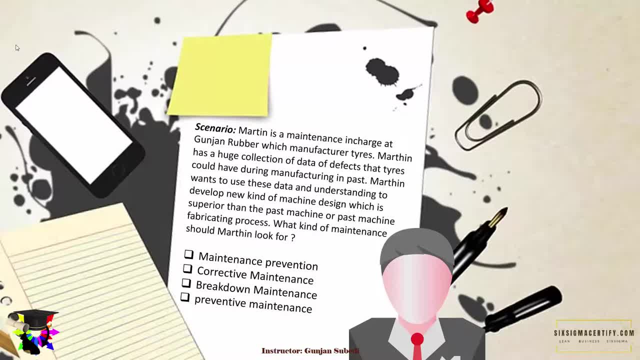 Fabricating process. What kind of maintenance is he looking for, Or should Martin look for? Is it preventive maintenance? Is it corrective maintenance? Is it breakdown maintenance Or is it preventive maintenance? Take your time to think. You can even pause the video now. 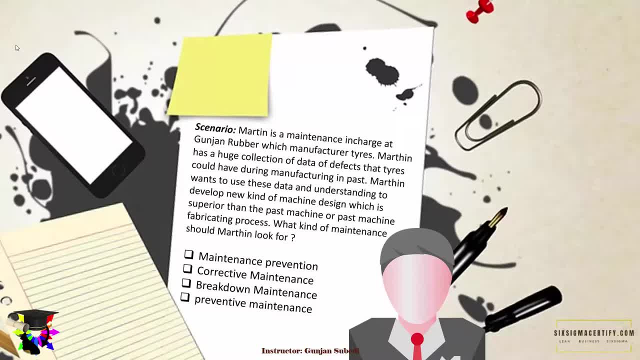 Okay, Let me tell you the right answer for this question, As Martin is trying to use historical data, or past data and experiences to improve the maintenance and operational efficiency of a new machine or new machine process in future. he is looking for maintenance prevention. 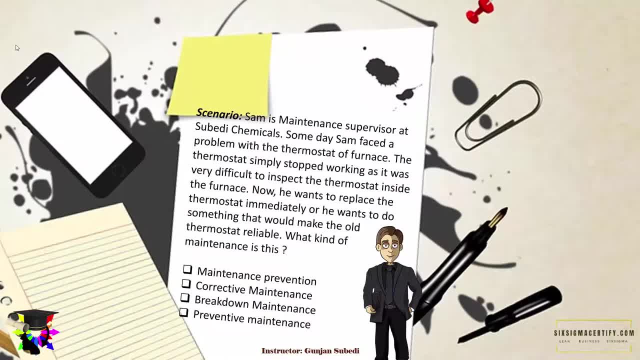 Okay, Let's see the second scenario. Sam is a maintenance supervisor. as Gunzen Rubber, He is a maintenance supervisor at Suezi Chemicals. One day Sam faced a problem with thermostat of furnace. The thermostat simply stopped working, also because it was very difficult to inspect the thermostat inside the furnace. 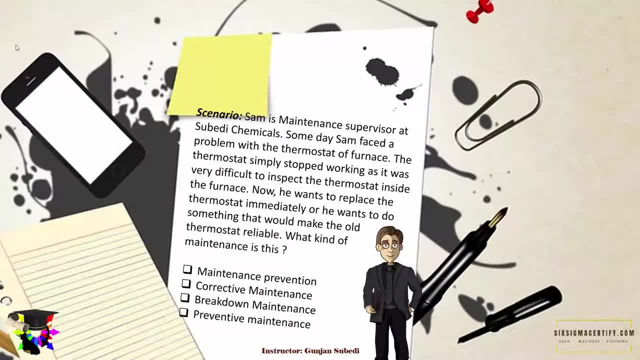 Now he wants to replace the thermostat immediately and he wants to do something that would make old thermostat reliable. What kind of maintenance is it? Is it maintenance prevention? Is it corrective maintenance? Is it breakdown maintenance Or is it preventive maintenance? Take your time to think. 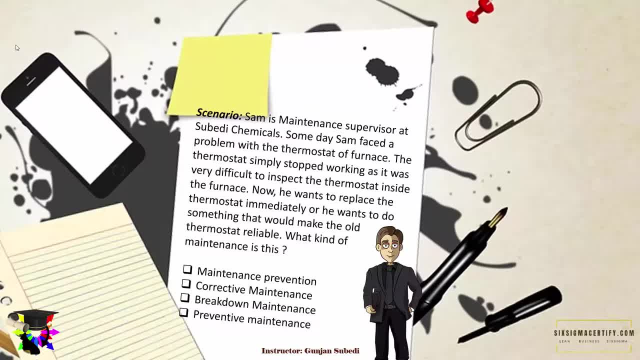 You can pause the video now. Okay, So the correct answer for this question is: it is the breakdown maintenance. In breakdown maintenance, we go for maintenance only after the equipment or part of the equipment breaks down, Which is not always a reliable and better option than preventive maintenance. 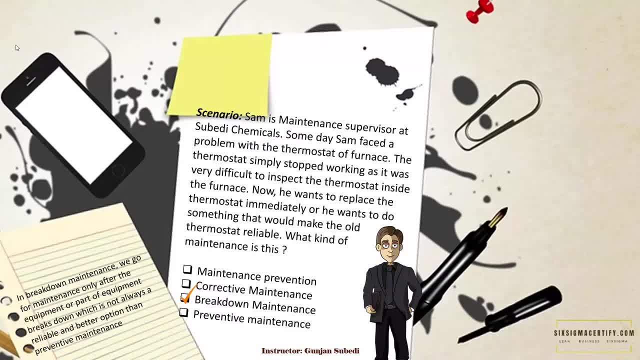 But nevertheless there are always one or many incidences of breakdown maintenance in any industry or any company.